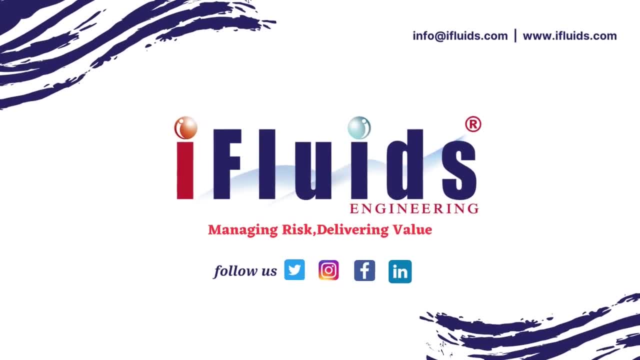 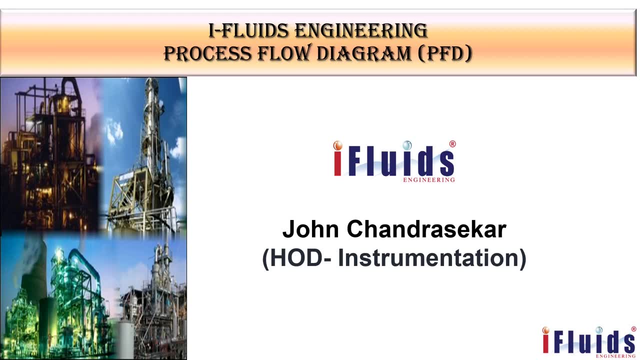 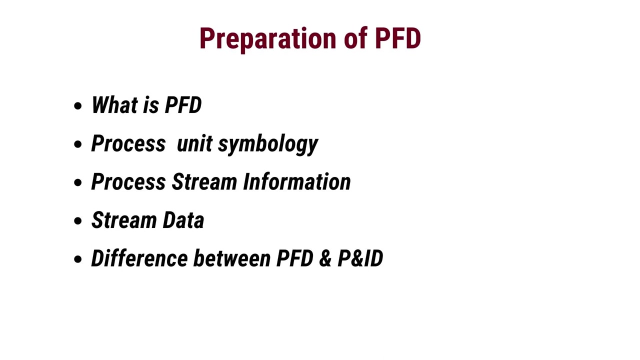 Good morning all My name is John Chandrasekhar. It's only instrumentation. Today we are going to discuss about process flow diagram preparation, How we are going to prepare the process flow diagram. There are five important things we are going to discuss. The first one is the what is process flow diagram, PFD. Second is: what is process unit symbology? What are the process unit symbology used in this process flow diagram? 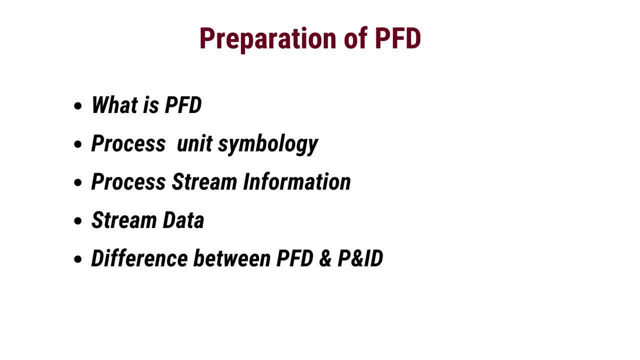 Third one is the process stream information. Different streams are in that process. So what are the process stream? how they are going to be noted in the process flow diagram. The fourth is the stream data. How will you show the stream data in the process flow diagram? 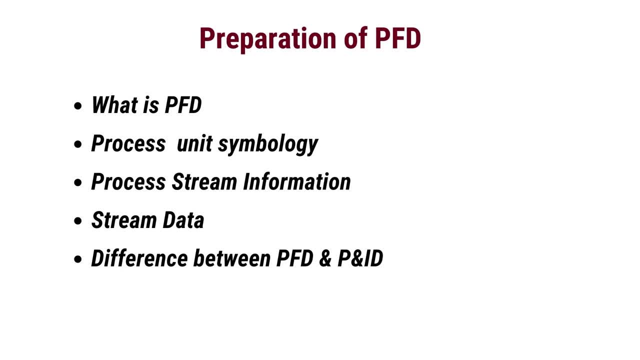 The final one is the difference between P&ID and PFD. You know what is P&ID: pipeline and instrumentation diagram. PFD is the process flow diagram That is in between. What is the difference between both? So we can move to the presentation. 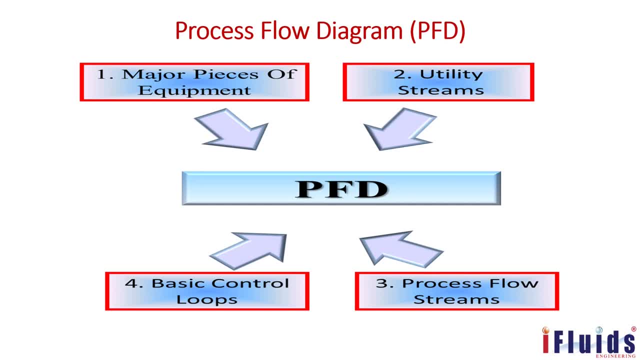 The process flow diagram. there are four major things are there. one is the major pieces of equipment. there are two types of equipments. are there the mechanical equipment? two types of equipment. one is a static equipment, another is the rotating equipments. static equipments are vessels, columns, heat exchangers that are static equipments. 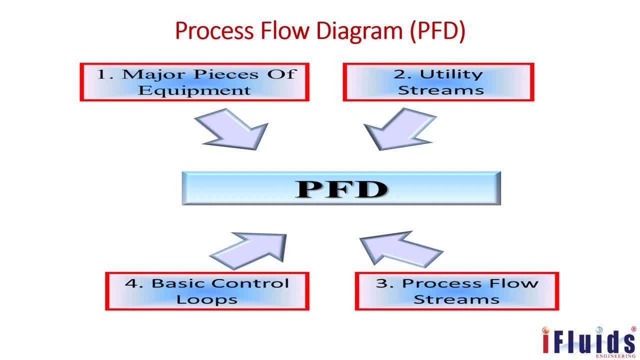 rotating equipments are pumps, agitators, compressors. that are these things. we are going to show the major pieces of equipment. the another is the streams, including. first you will eat steam. you have to show here instrument, here water cooling water steams, high pressure steam, low processing nitrogen, all utility schemes we have to show in the ft. then process frosting process. 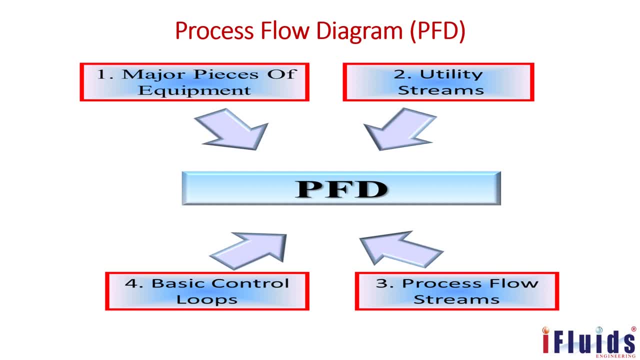 further scheme is the feed, ethylene feed, crude feed, maybe it is a another chemical line so that process protein streams we have to show. the last one is the basic control loops, the important loops- feed forward control, feedback control, ratio control- that we are going to show in the 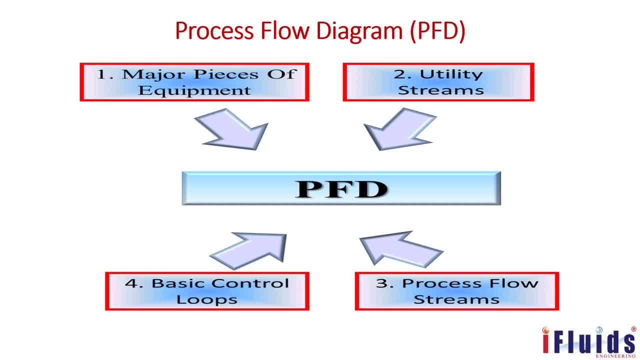 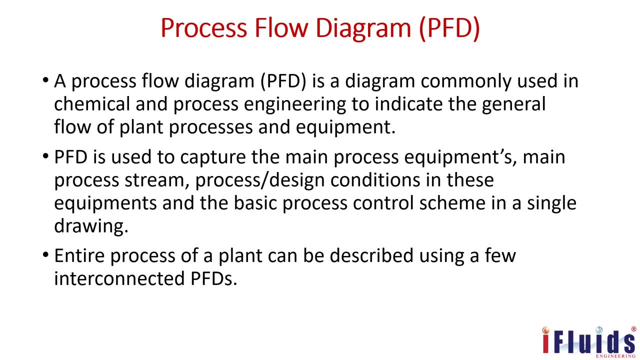 pft: minor lines, minor streams, small small lines. we are not going to show in the pft. a process flow diagram is a diagram commonly used in chemical and process engineering to indicate the general flow of plant process and equipment. pfd is used to capture the main. 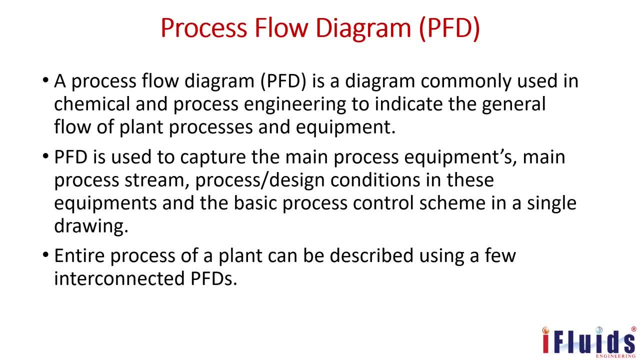 process equipments, main process stream, process design conditions in these equipments and the basic process control scheme in a single drawing. entire process of your plant can be described using a few interconnected pfds. as i already told, pfd is used to capture the main process equipment, static equipment and rotating equipment. 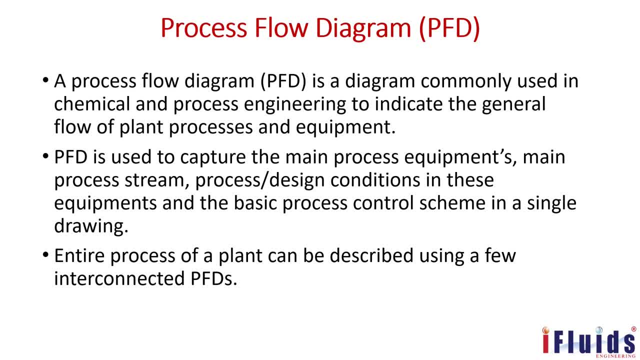 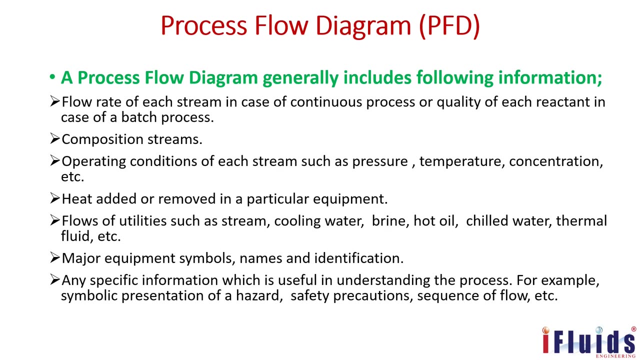 and main stream and utility stream. some basic design conditions. for example, if you show a pump, what is the pump capacity? maximum pump capacity, maximum pressure, maximum flow. design conditions we are going to show in the pft. a process flow diagram generally includes following information: flow rate of each stream in case of continuous process. 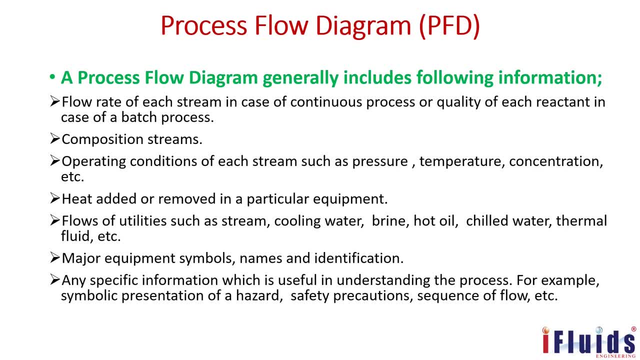 or quality of each reactor. in case of batch process, there are two types of process. one is a continuous process, other batch. in case of continuous process, the stream flow rate we have to show, in case of batch process, how much reactor we are using, quality or quantity of the 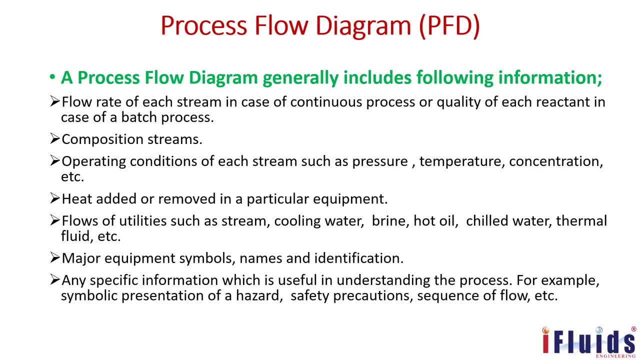 reactor. the composition of streams. some streams can be two compositions, maybe water and crude, or maybe it's hydrogen nitrogen, like like that some streams. composition will be there: air and fuel ratio, then operating conditions of each stream, such as pressure, temperature, concentration, etc. so operating conditions: there will be two types of. 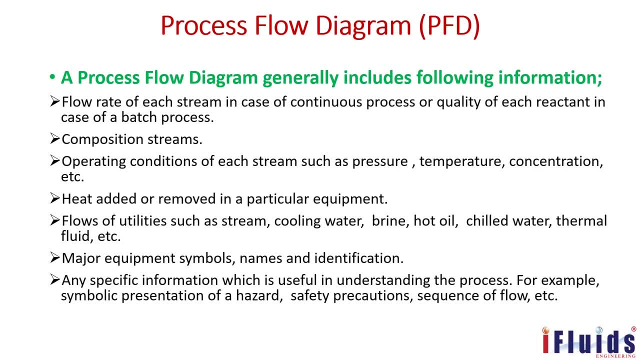 conditions will be there, one design conditions, another is operating conditions, operating pressure, temperature, flow level. all basic parameters we have to show in the pft, heat added are removed in a particular document. if, in case of you are using a distillation column in our heat exchanger, how much heat is added? how much it is? 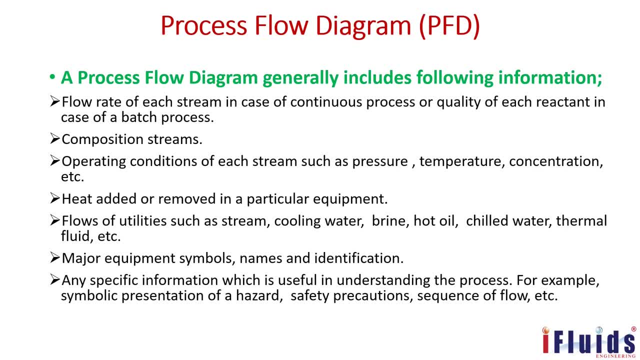 removed from there. even in case of cool coolers it is removed. in case of heaters it is a heat added, so that information we have to capture in the pft flows, flows of utilities such as stream cooling water, brain hot oil, chilled water, thermal food, etc. as i already informed, all utility stream. 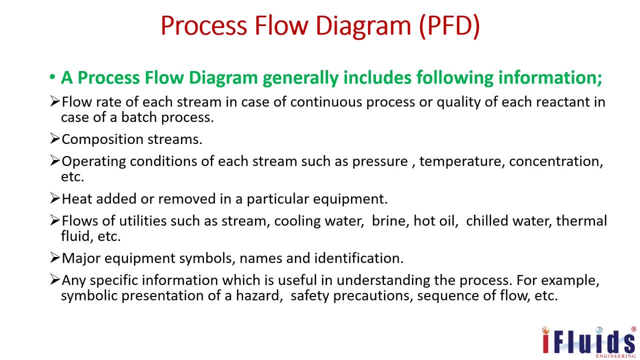 water, cooling water, nitrogen, oxygen instrument here, whatever fuel gas. so all flow flows should be mentioned in the pft. then major equipment symbols, names and identification. i already discussed these major equipments, static equipment and rotating critical equipments. their name symbols we have to use and their names also we have to. 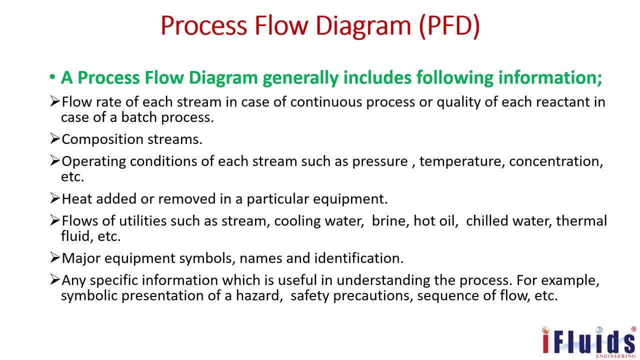 put then identification. identification is that to check the flow that we want to follow. these are called pft, so this is a simple instruction to check the flow of air flow process. that's how you can use the pft and this is a simple instruction if you have a pft or you want to check your pft. 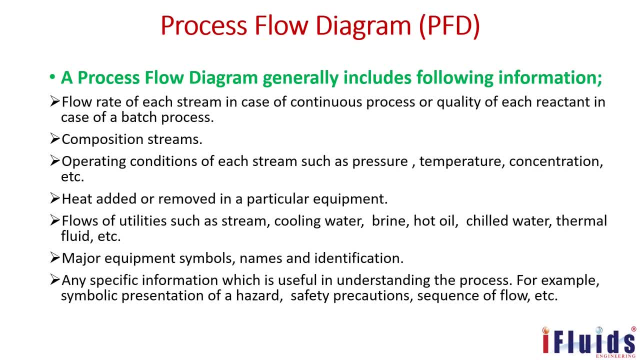 you need to know that. what is this? pft is like. this is a pft, which is the pft. that is the pft in case of we are using these pft. we may not use it as a pft, but we do need to be able to. 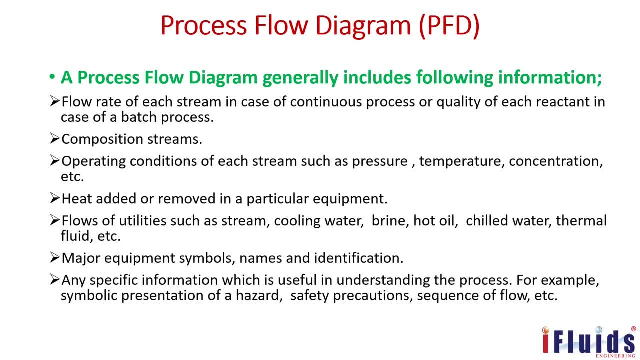 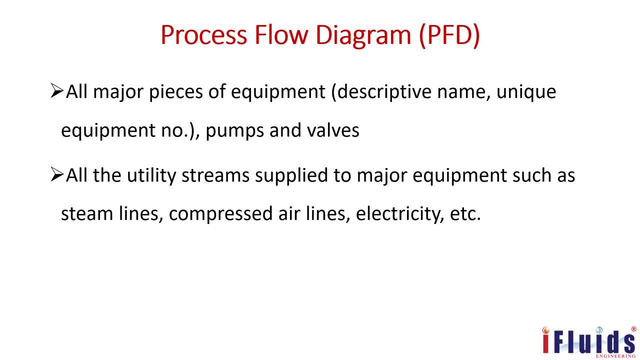 use them in a specific way. it is the same process. All major pieces of equipment, descriptive name, unit equipment number, pumps and valves. there are pumps and valves, also rotating equipment. that major valves. we have to show Minor valves, minor isolation valve. we don't need to show in the PFD All the introductory streams applied to major equipment such as stream line number, stair line, electricity should be noted in the PFD. 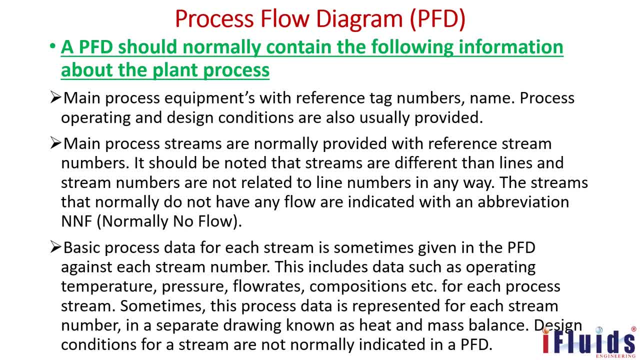 A PFD should normally contain the following information about the planned process. Main process equipment with reference stack number, name, process, operating and design conditions are also usually provided. Main process streams are normally provided with reference stream numbers. There should be a stream number. Each stream has the number One input to the column, distillation column or heat exchanger. 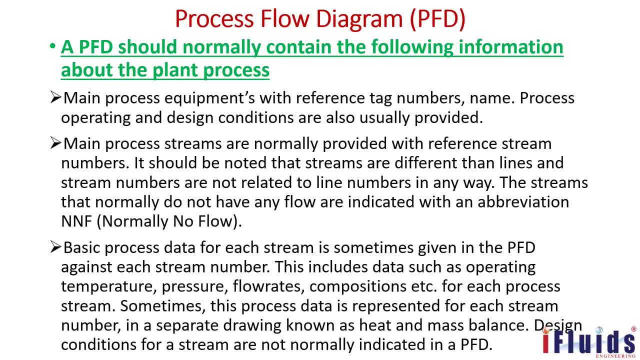 One input stream should have the number Reference stream number. It should be noted that streams are different than the line numbers. We should have clarity. If you go to P&AD, process, piping and instrumentation diagram, there will be a line number. 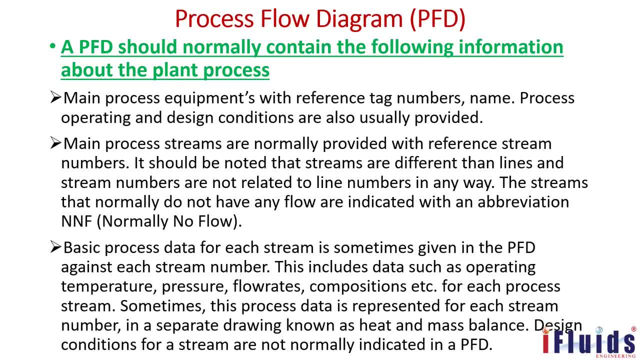 But here line number will not be there. Line number is different from the stream number. Stream number is different from the line number, The stream that Normally do not have any flow or indicated with the abbreviation Normally no flow. Some stream may be having flow during the startup, Maybe intermediately it will flow. Normal operation: it will not flow. 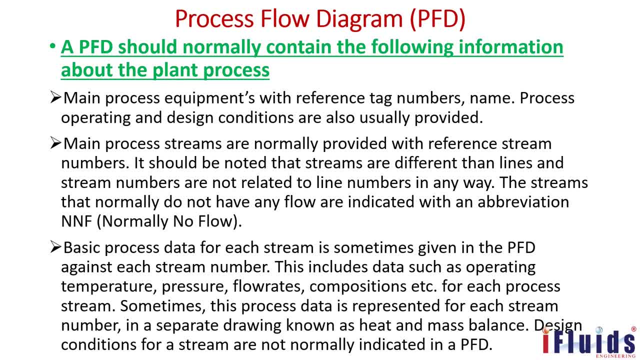 That case you have to put N, N, F. Normally no flow. That indication we have. Basic process data for each stream is sometimes given in the PFD, again each stream number. This includes data such as operating temperature, pressure, flow rate. 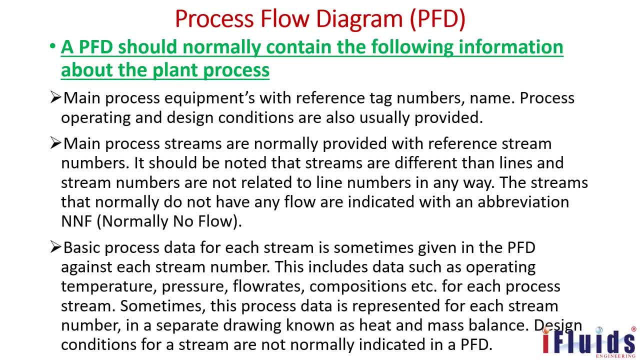 Composition, etc. For each process stream. sometimes this process data is represented for each stream number in a separate drawing known as heat and mass balance. Design conditions for a stream are normally indicated in a PFD. It is nothing but each process conditions of a stream. you have to put it in each stream. 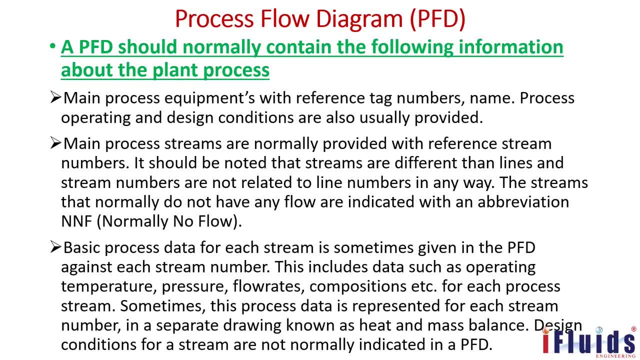 But if it is required, you have to add a tabular column, You have to add, You have to add a tablet column: stream 1, stream 2, stream 3, then what is the operating pressure, operating temperature flow, then stream 2, operating temperature flow level. like that you can add a. 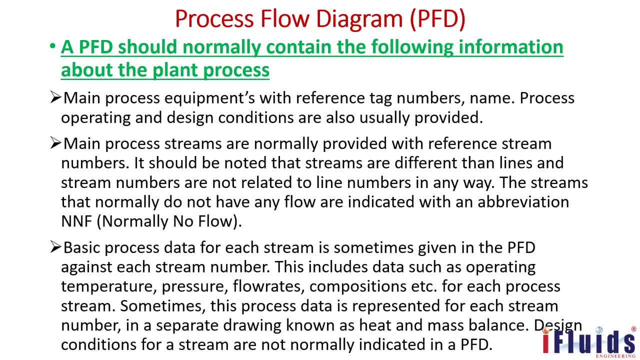 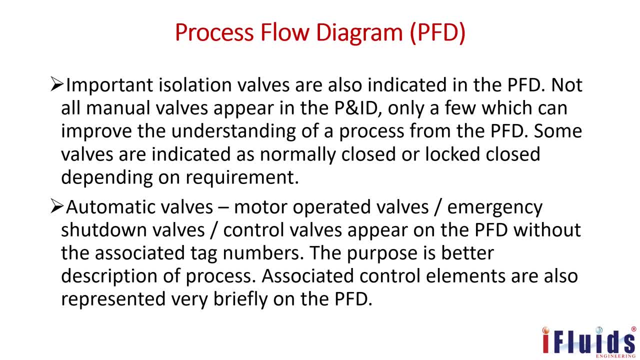 one separate tablet column. i can show the tablet column later slides. important isolation walls are also indicated in the pmd. not all manual walls appear in the pmd, only a few which can improve the understanding of process from the pmd. you have to show the all important walls, all control. 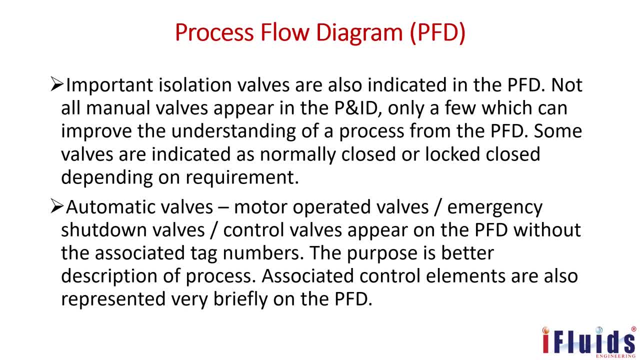 wall, shut down walls, even manual isolation also it is a very big wall, important walls now small, small isolation walls and drain walls. in order to show some walls are indicated as normally closed or locked closed, depending on the equipment requirements, you have to show the normally open, normally close. also that we have to show auto putting was, motor operated was. 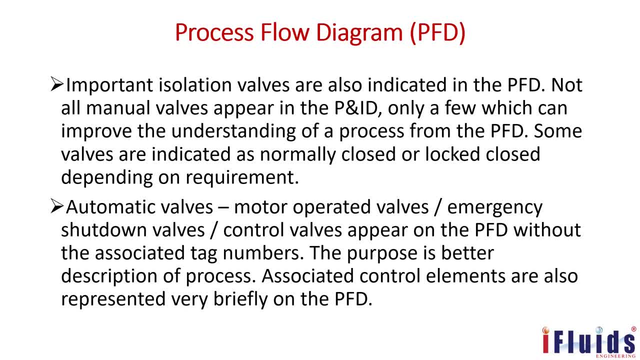 emergency shuttle walls. control walls appear in the pmd without the associated tag numbers. you don't need to put the tag numbers. tag numbers will be in the pin. only here you can show pcb pressure control wall, fcv flow control wall like that only. the purpose is better description of process associate. 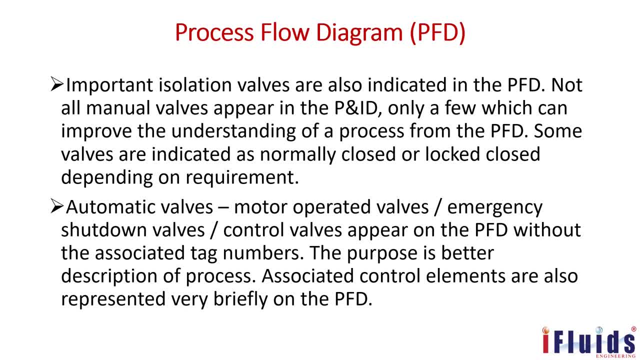 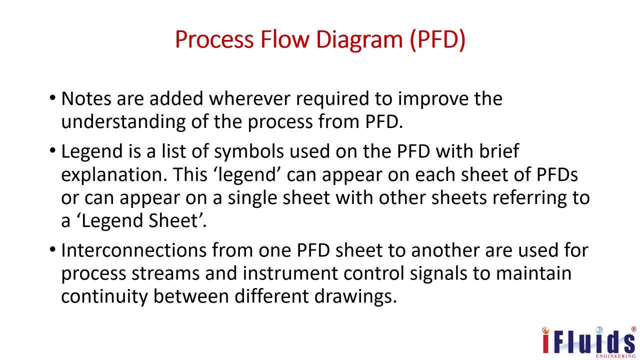 control elements are also represented very briefly at the pmd. sometimes if you want to show the control loop, control loop, maybe one control one, one transmitter and one plc or dcs, that loop we can show here. it is required to understand. then you can show here. notes are added wherever required. 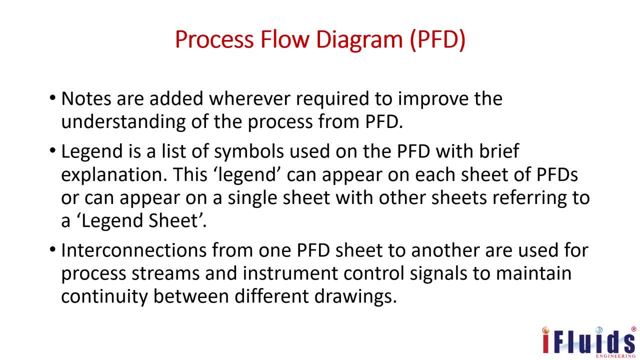 to improve the understanding of the process from pmd. you can put a note wherever you want to explain more information, give more information. you can add note, small note. this stream is from this vessel. this is going to that column. like that, small notes, you can put it. legend is a list of symbols used on the pfd with brief explanation. this legend: 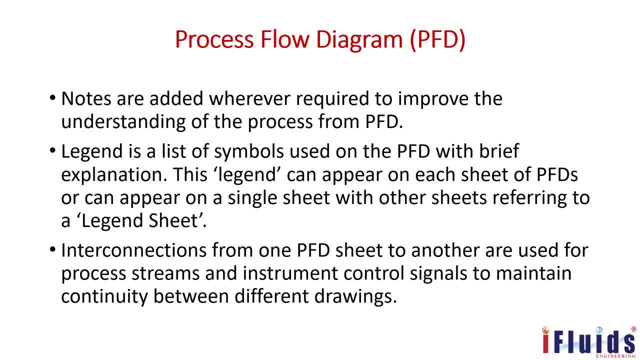 can appear on each sheet of pfds or can appear on a single sheet with other sheets referring to a legend sheet, legend legend. what are the symbols we are going to use? that legend you have to mention in the each sheet. for example, pfd. first pfd, we used some columns or exchangers or pumps. that legend you have to. 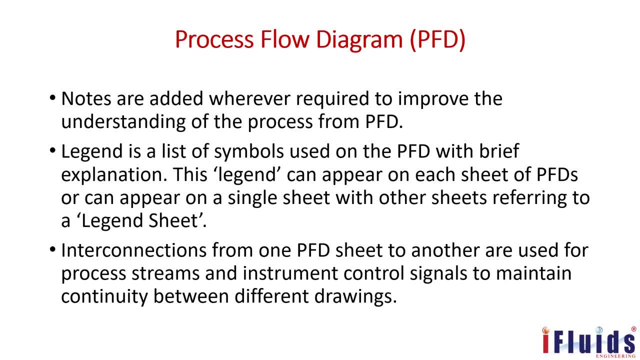 use the same sheet. otherwise, if the number of legends are more, you got to prepare your legend sheet. okay, the legend sheet. then you have to show the reference. please refer the legend sheet numbers also like that interconnections from one pfd c2 another are used for process streams and instrument. 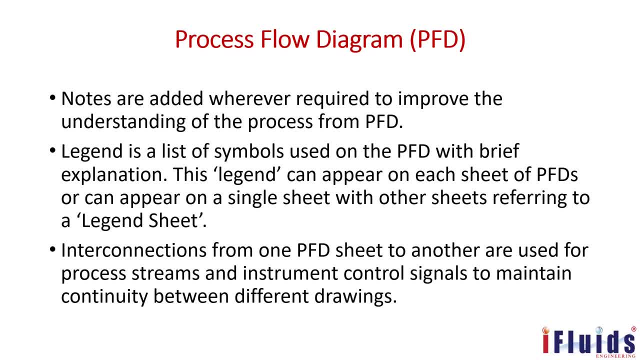 maintained continuity between different coils. in case of two, three pfts are there from one pfd to another pfd. if the stream is going you have to show the interconnection from two. similarly, the for instrument signal also, maybe the flow meter will be in one pfd control volume. 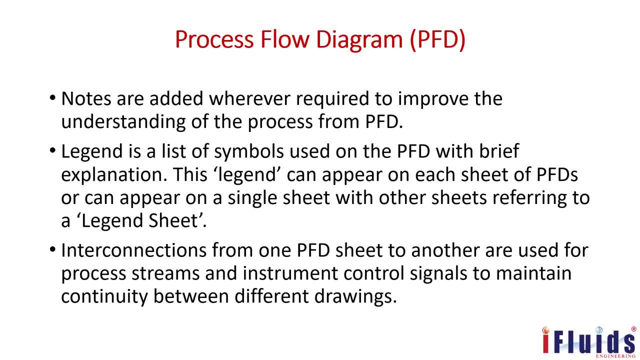 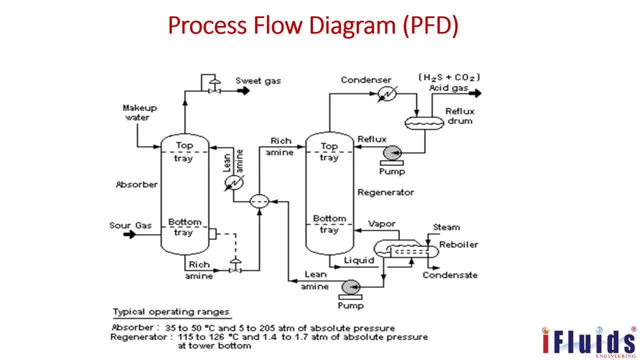 may be in another pfd, so you have to show the signal flow from this pfd to another pfd. this is one example, small example, of process flow diagram. there are two discussion columns, are there? uh, one is observed. basically it's: one is observer and that is a regenerator. 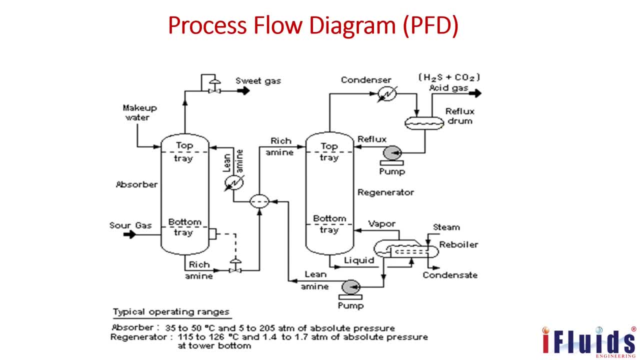 uh, the showcase. showcase is the feed. that is called stream. okay, make up water. the top that is a utility stream. i already told you have to show the main process: stream all the way to the top. so utility stream also. it is called observer. that's why it's the observer name is there. 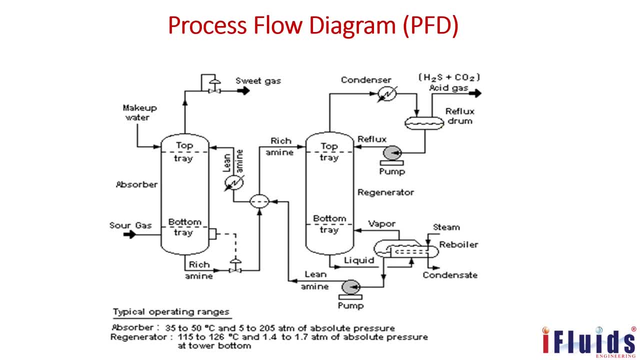 then the outlet is going to one exchanger, heat exchanger, then it's go to another regenerator and pumps are there, reflection elements are there. so utility and major streams we have shown in the major equipments also, for example, this observer and regenerate is the equipment static equipment? okay, this heat exchanger is a static equipment, condensator is a static equipment. 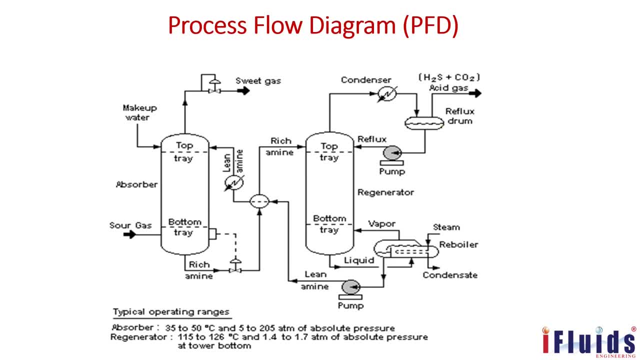 reflux drum is a static equipment, but the pump, the pumps, are rotating equipment. then major wall: in sweet gas line there is one wall. so here in rich amine line, also, one control wall is there. so level control wall is there. the important walls we have shown here. okay, some operating. 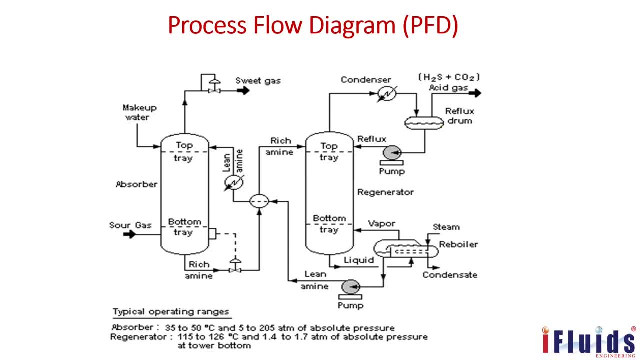 ranges already told. we have to mention the operating the below that, 35 to 50 degree and 5 to 205 atmosphere pressure. so like that we have to important parameters. we have to show in that one. these are different symbology, unit symbology, i told. 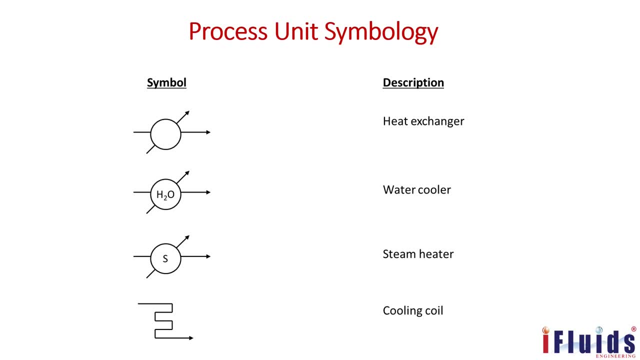 her that heat exchanger, water cooler, steam heater, cooling coil. if it is a water cooler, h2o inside, you have to write h2o inside. if it is a steam heater, yes, should be inside. if it is a some other heat exchanger, then it would be a common heat exchanger. 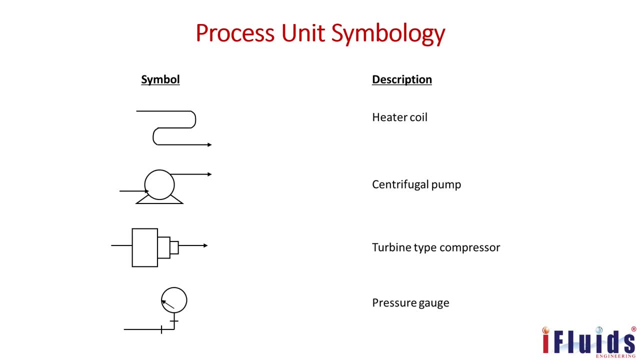 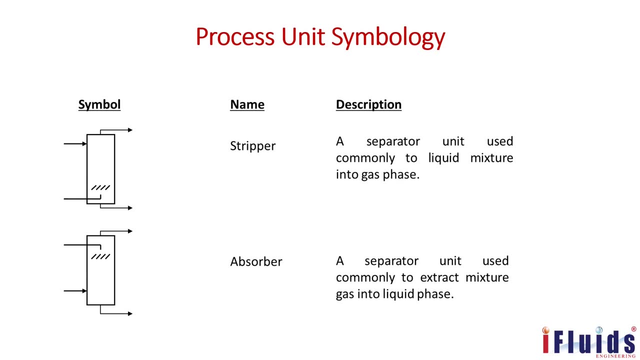 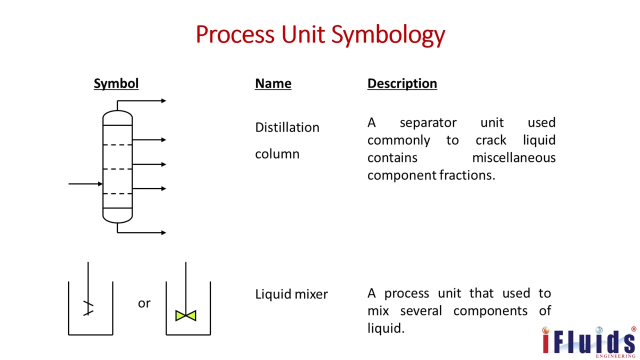 then the heater coil: centrifugal pump, turbine type compressor pressure cage. this is the stripper and observer. observer is: from the top, you have to spray something. stripper, from the bottom, you have to strip it. this is the distillation column, a separator unit used commonly to crack liquid. 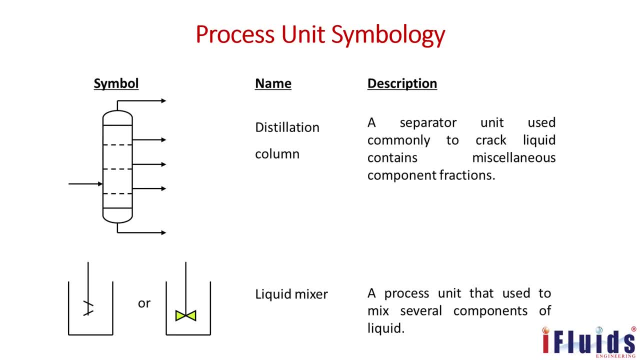 contains miscellaneous convert fractions, then liquid mixer, a process in it that used to mix several components of liquid. both are liquid mixer only. the difference between first one and second one is it having only one blade liquid mixer that another one have different levels. different blades may be there to mix the 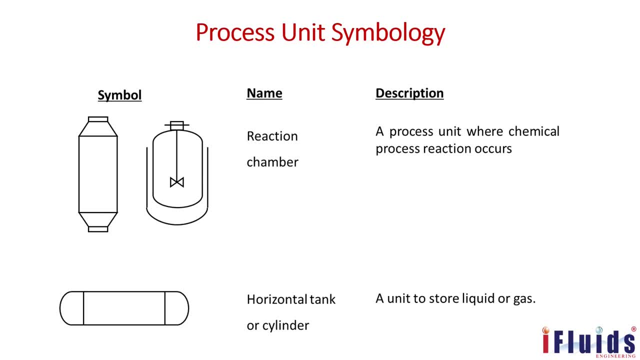 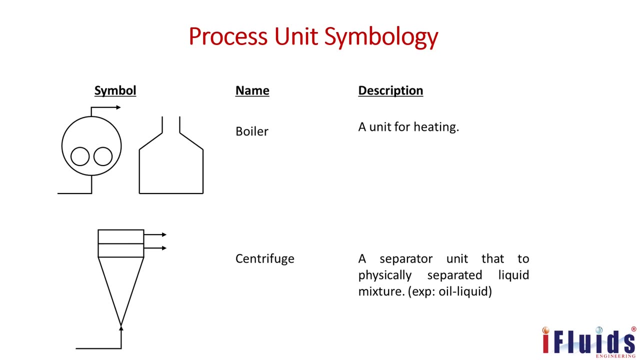 liquid, then this is a reactor chamber. two different type of chambers are there then: horizontal, tank or cylinder. these are the symbols we are going to use in the uh pfd. this is a boiler. the boiler is the side. first symbol is a side view, another is the 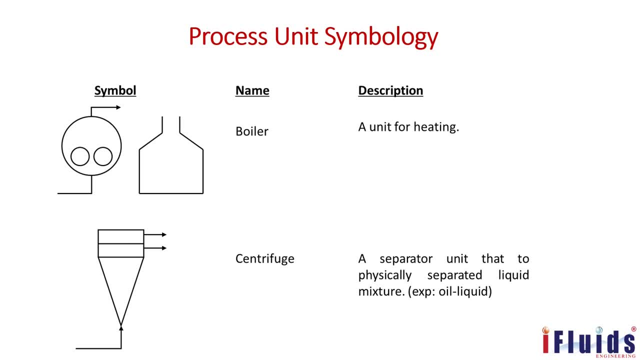 symbol- boiler symbol. when you are going to show the fuel- gas and air- boiler air- then the side view, that two circle, small circle that you have to show when you are going to show when a liquid is boiled, then that will you have to show: that hot water top. 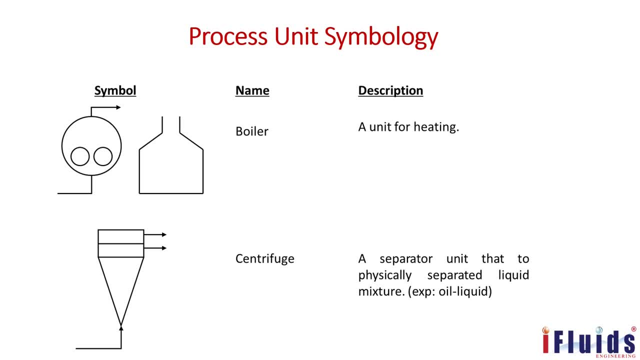 you have to show when you are going to show the utility, it will reduce the fuel gas, as the utility instrument here or other things are, um or smoke is coming out that you are going to show. then that first symbol. the another symbol is for process. okay, then this is centrifuge. 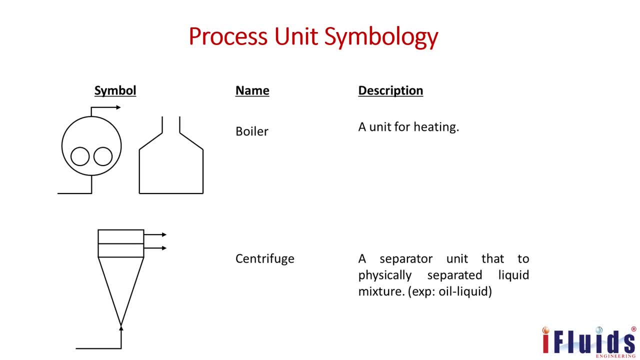 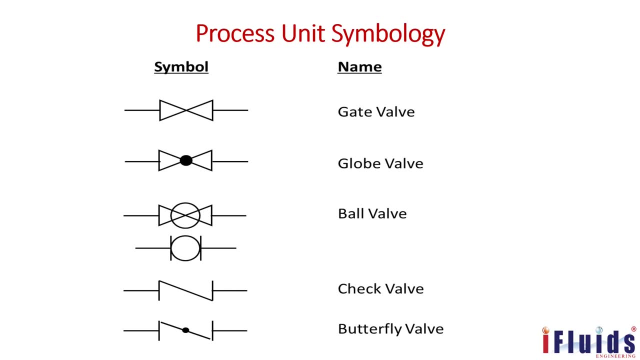 centrifuge is nothing but your rotating equipment. you have to centrifuge with the gravity. you have to centrifuge separate two liquids. this is the gate wall symbols. different type of walls: globe wall, gate wall, globe wall, ball wall, check wall, butterfly wall. so you have to see the difference between each wall. 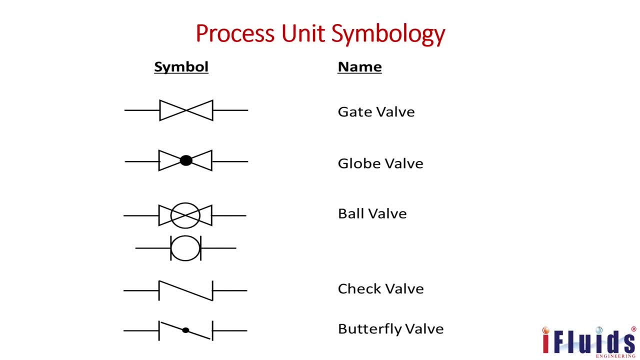 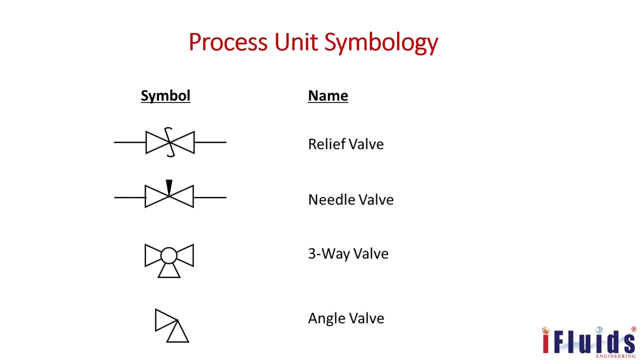 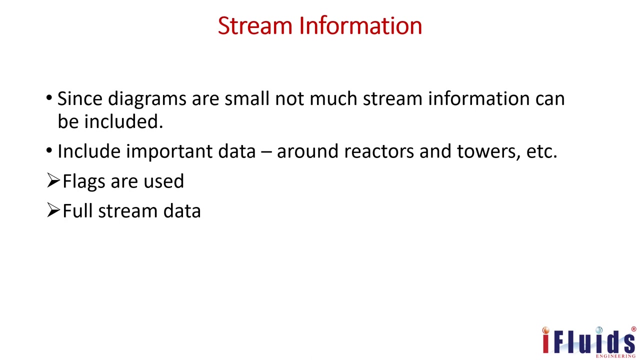 check wall and butterfly wall looking similar, but there will be one small uh dot in the center. it's a pivot. actually it's a butterfly wall. this is a relief wall, needle wall, three-way wall, angle wall. since pfd diagrams are small, not much stream information can be included, since pfd is a primary basic diagram. 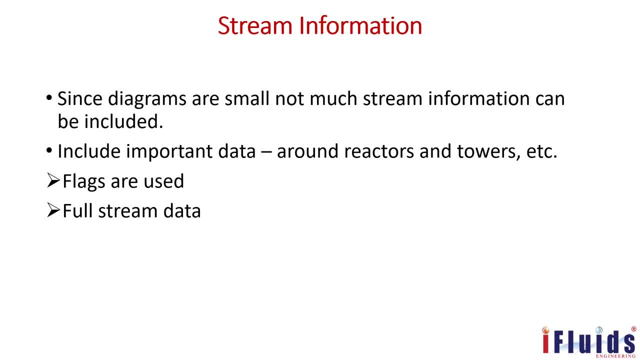 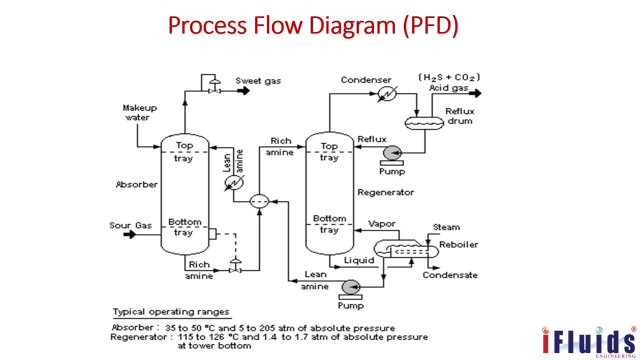 for the process. you cannot put all the stream information. the previously we have put the stream information, see the bottom. only here what you have put it: temperature and pressure only. but if you want flow, if you want level, if you want density, viscosity, all information you cannot put in the bottom. 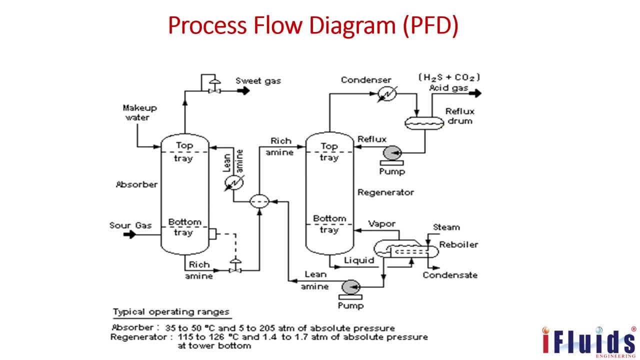 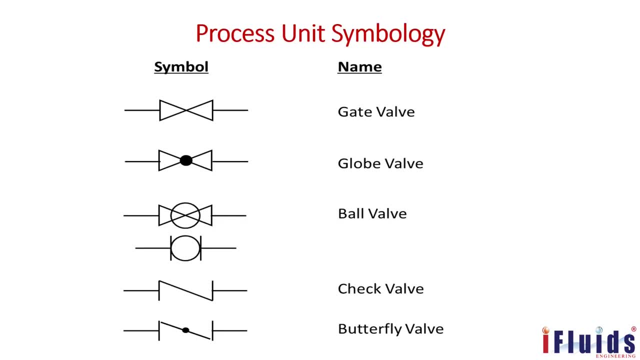 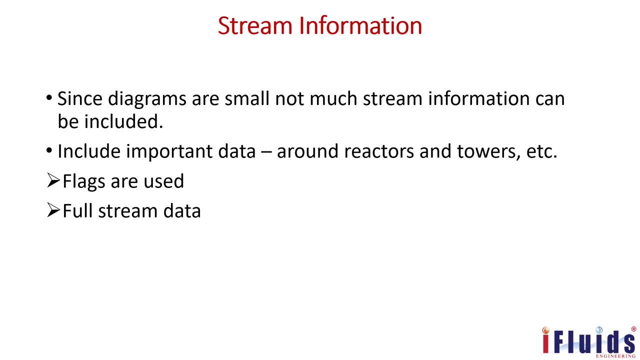 one stream. you can put: if here, if it is five streams are there, then five, six parameters are there. you cannot put in the down. that's the way here we mentioned. since diagrams are small, not much stream information can be included, include important data around reactors and towers, etc. 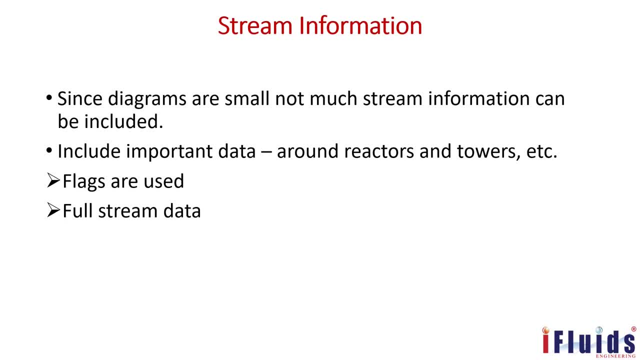 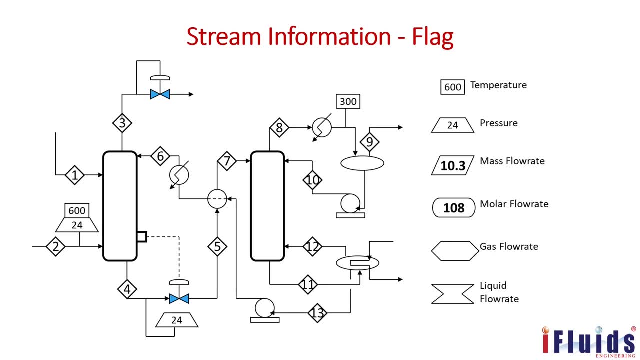 flags are used, full stream data, flags and full stream data. what is flags? what is full stream data? the next slide we are going to discuss- see. this is a flag 600, one rectangular in the right hand side, if you see. 600. temperature, 24 pressure, 10.3. mass flow rate, 108 molar. 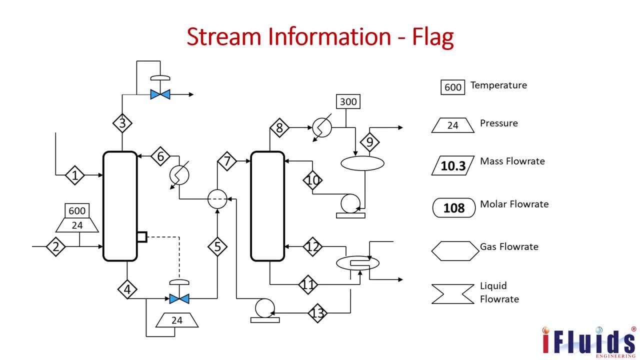 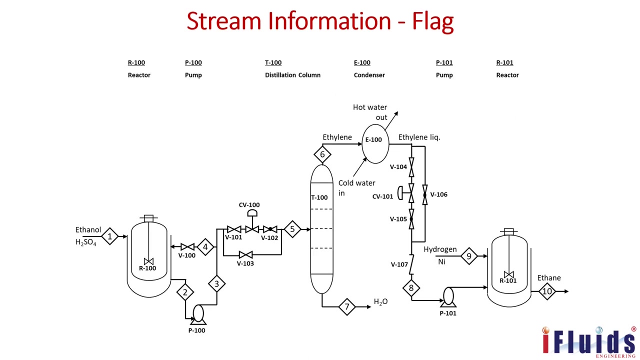 flow rate like that. this flag is used for the system. so if you have a stream number 2, if you have a stream number of a stream number 2, then you can use flags. you can use it where over 24 is there right hand side. if you see the stream number two, stream number two right hand side- 24 and 600. 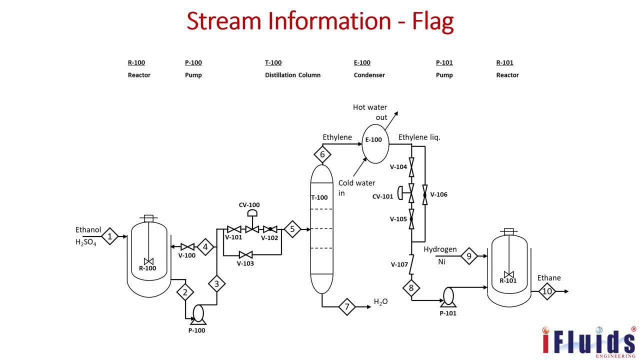 Here you can mention the name: ethanol and H2SO4.. Ethanol and H2SO4, you are adding to a reactor. Okay, So reactor is R100.. The reactor symbology, the top. you have to mention the reactor name and the number. 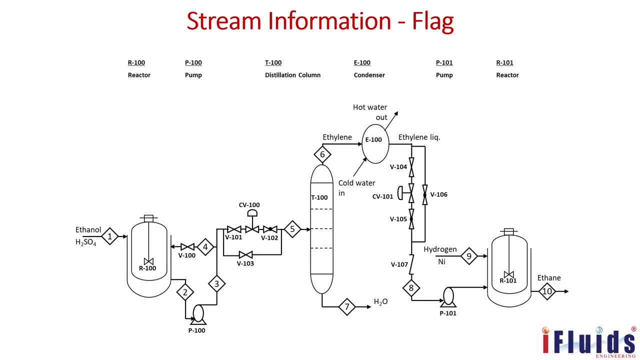 It's not a tag number, It's a number. Tag number may be different. Okay, In the P&ED you can mention the tag number. Okay, That may be tag T, dash R001.. Like that, maybe it's a different symbology. 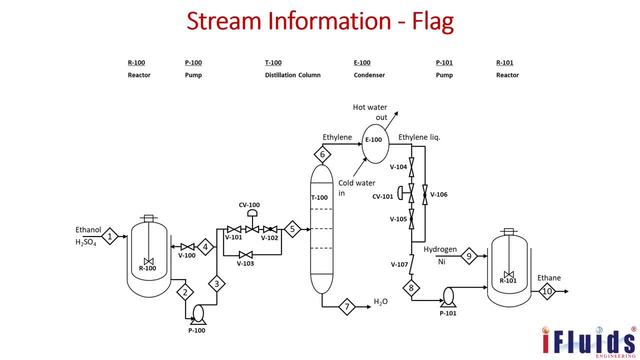 So you can use this information stream, information with a flag. Okay Here. 1 is first stream: ethanol and H2SO4.. 2 is the bottom. 3, 4,, 5,, 6.. Like that, up to 10.. 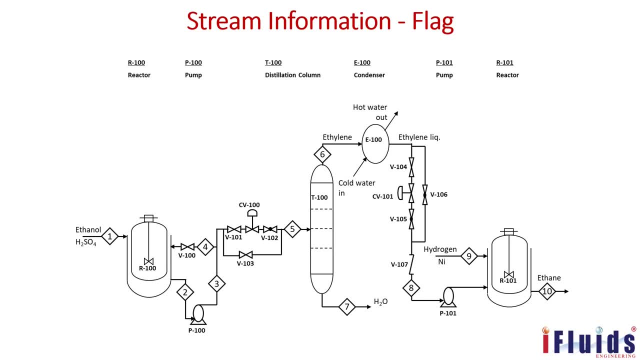 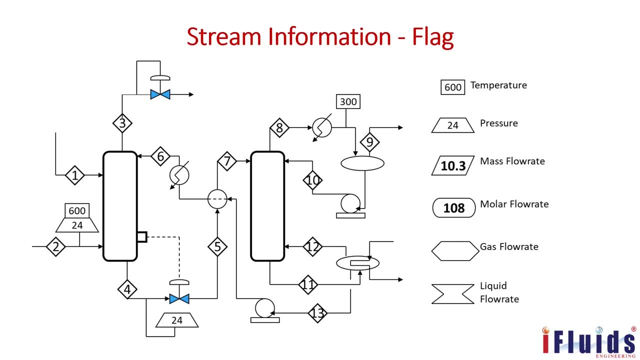 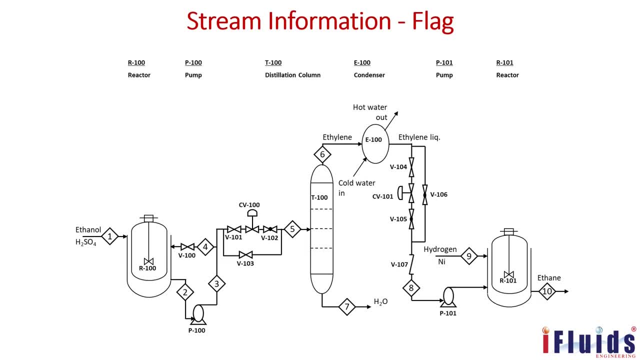 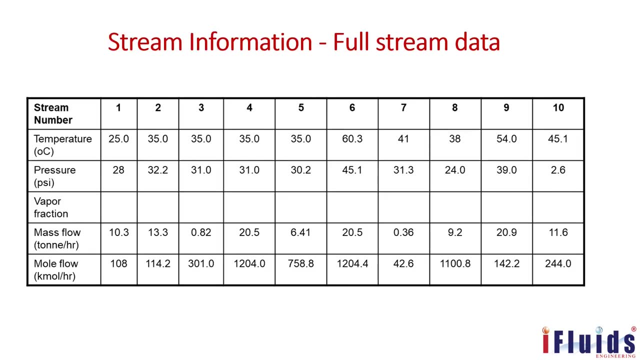 This is the process parameter flag. Here. it is a stream flag. Okay, Now see, This is a full stream data. As already I told, if it is small information, you can put in the below in the FPFD. If it is more information required, more streams are there, then you can add a separate table. 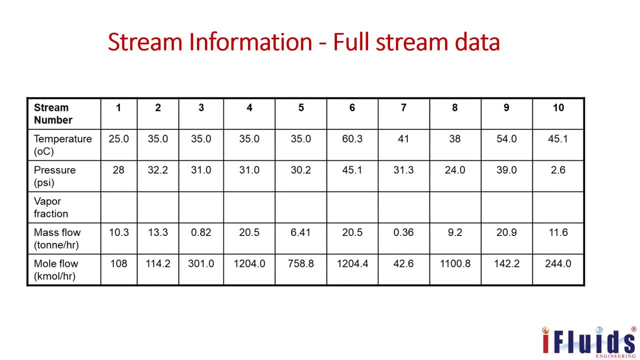 See 1 to 10.. 10 stream are the steam number one, two, three, four, five, then temperature, pressure, vapor fraction, mass flow, mode, flow. all information captured here of the all 10 streams, okay, okay, now you understand what is stream number and all basic parameters, important parameters captured in that table. 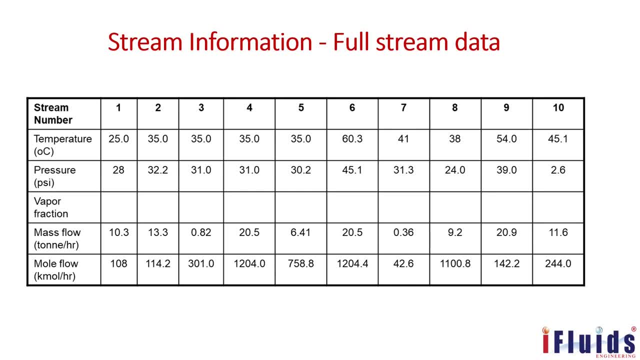 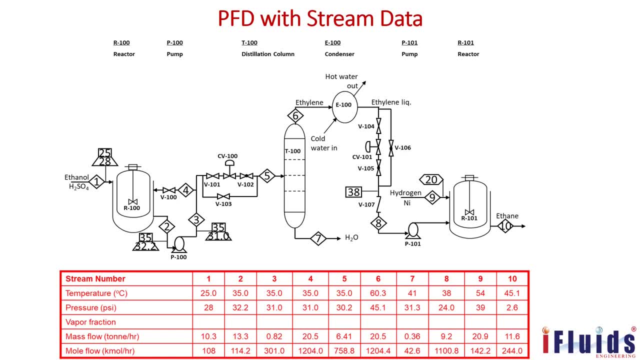 this table can be showed as a separate pft sheet or below the pft pfd stream data. if you have a sufficient space is there. you can show the table below the pmd. if it is better, always better. you keep the table below the so that you can easily correlate. 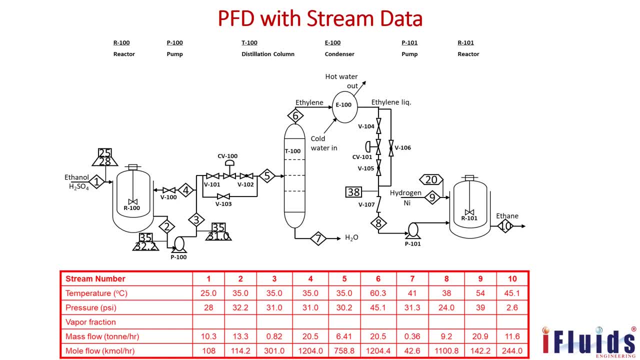 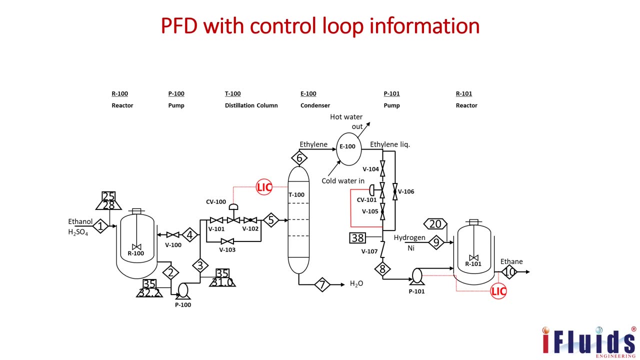 what is stream mode? what is the parameter? or is every time you have to go to the separate sheet and refer? but if it is more streams, more than 10, 20, then you have to keep a separate sheet. okay, now pfd with control loop information. already i discussed, told in some basic information, control. 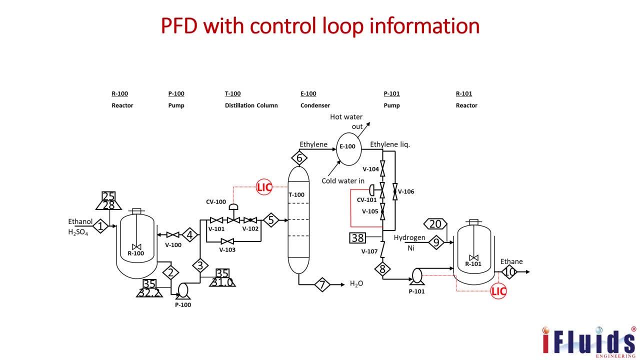 loops we have to mention here. one level control loop is the two control groups are there, see lac. here. on lac in the t contact distillation column 101, lac is there, cv 100 is there. there you are going to operate one pump also, p101, and one more cv 101 is there. so these are the basic important loops. 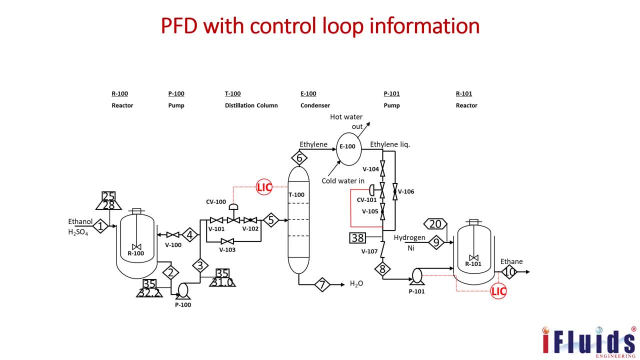 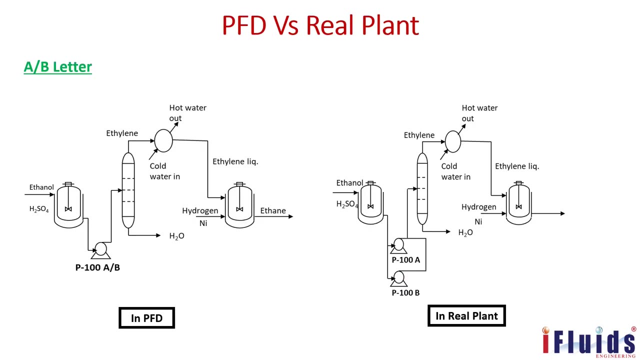 we have to show in the pft. so in the nutshell, pfd, we have to show the static equipment, rotating equipment. flags- you can use it. stream numbers: you have to use it. steam parameters as a table- you can use it. then important loops you can show okay. 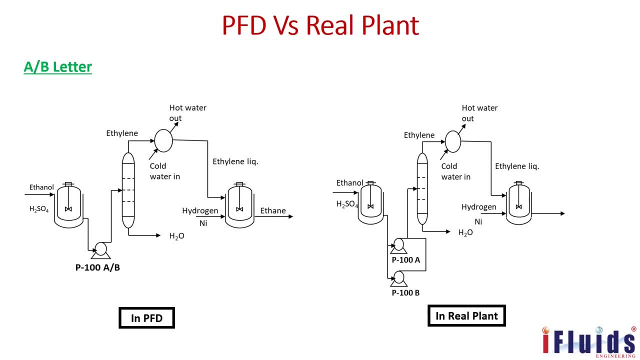 this pfd is real plan. so in the pfd you have to show two pumps as a p100, a slash b. the left hand side is a pfd but the real plan in the right hand side. okay, if you go to real plan, the pump will be. 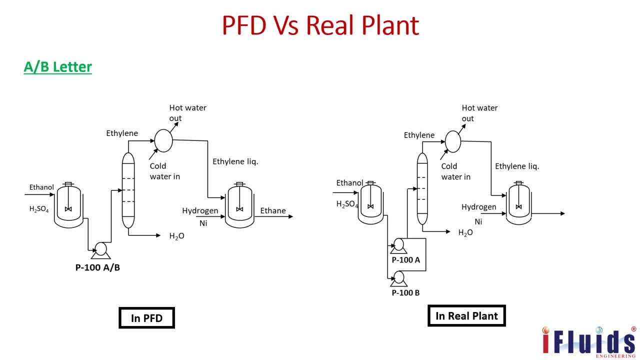 different, see 100a, 100b is it showed different but if it is in the pfd. so, as i discussed, pfd in in the plant, showing the PFD is different from the real plant, The PFD, the pumps, two pumps: A, B. 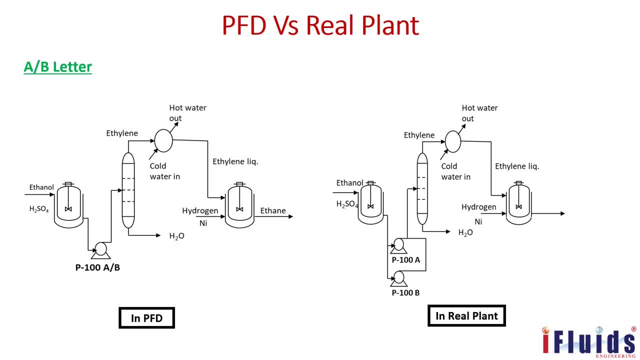 in case four pumps- A, B, C, D- you have to show under A, slash B, slash C, slash D. But in the real plant, even in the P&ID, you have to show all the pumps. That is the difference between the PFD verse and real plant. 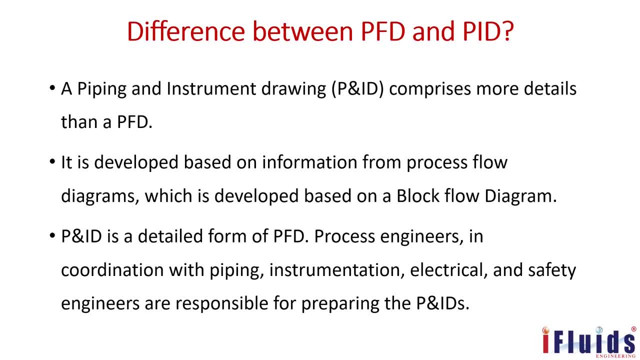 The difference between PFD and P&ID. A piping and instrument drawing comprises more details than a PFD. It is developed based on information from process flow diagram, which is developed based on block flow diagram. There are two types of process diagrams. One is 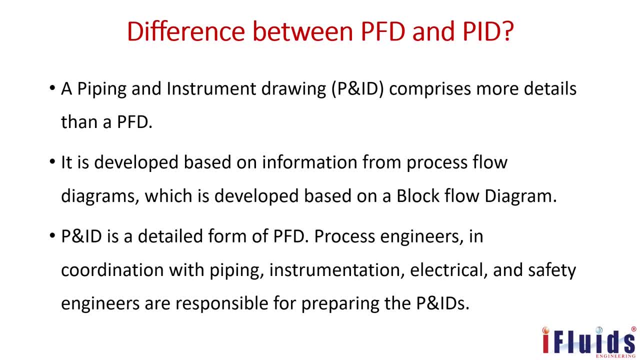 block flow diagram and it is a process flow diagram, PFD. But PFD is the mother document for the P&ID. P&ID is a detailed form of PFD: Process engineers in coordination with piping instrumentation, electrical and safety engineers.